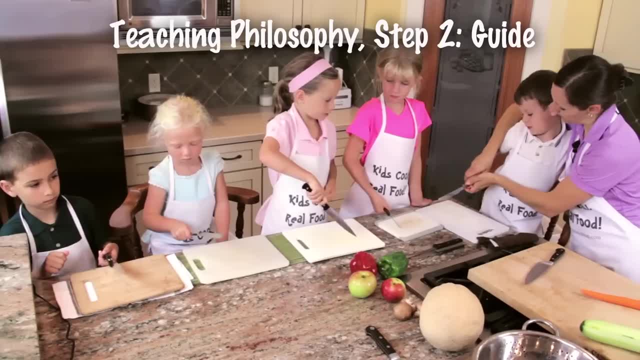 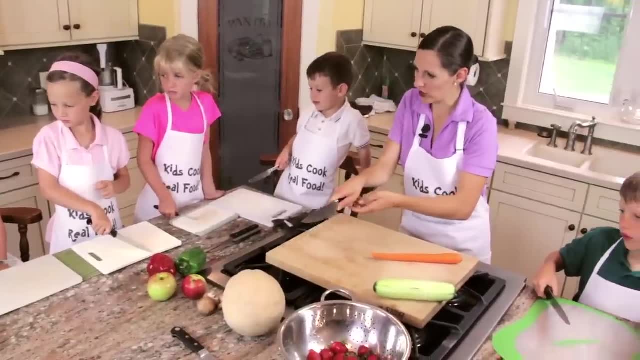 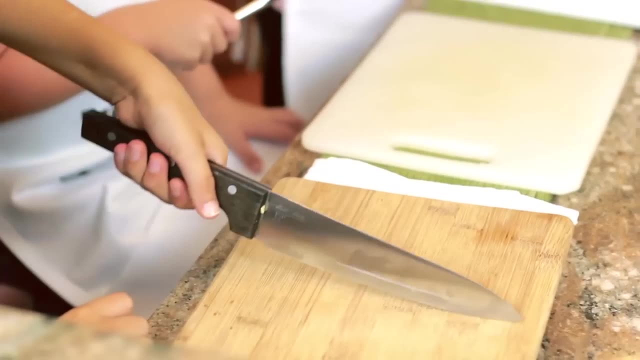 on top. Let me show you Turn it just a little like that. Very good, Yep, there we go. Quinn, turn your thumb around a little bit so that your hand- yeah, your hand- needs to be on top, because that's where you get all your muscle pressure pushing down to do things. 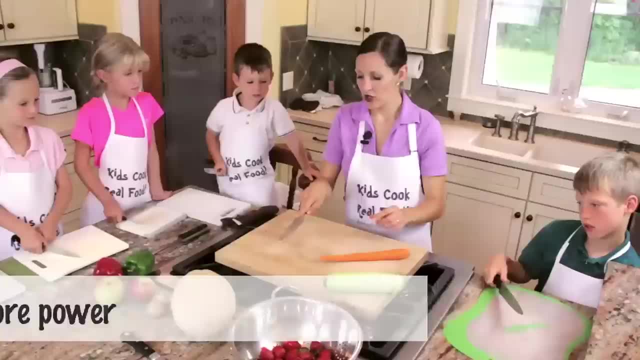 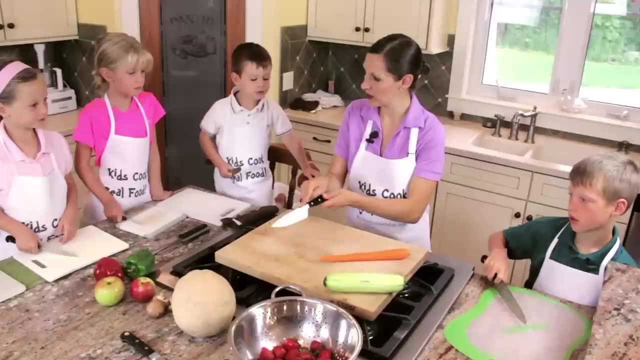 If you need more power, if you're trying to cut something, and it's tricky, don't put your finger down the knife. It's not actually going to give you very much more strength. What I want you to do is move your hand up closer to the knife. It's called choking up. You can move it up. You can even. 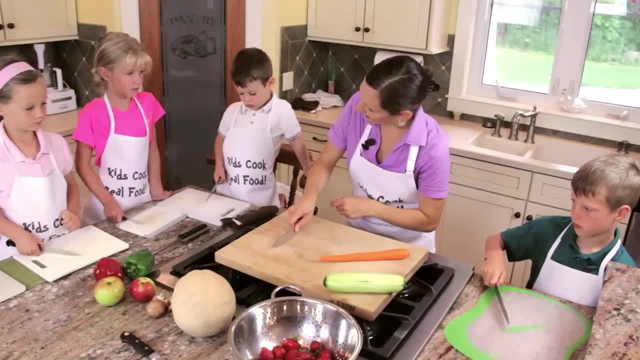 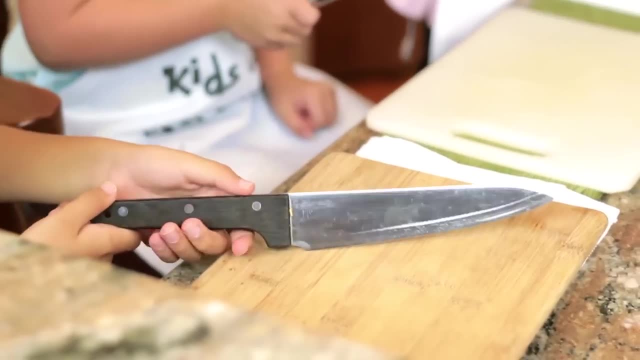 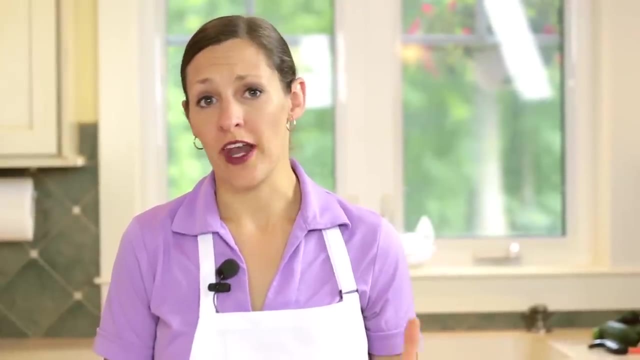 put two fingers on the sides of the knife like that, and then you'll get enough strength. So, Quinn, can you show me how you might choke up, move your hand up closer and get that thumb wrapped around? Yep, there you go. All right, here's a super important rule that. 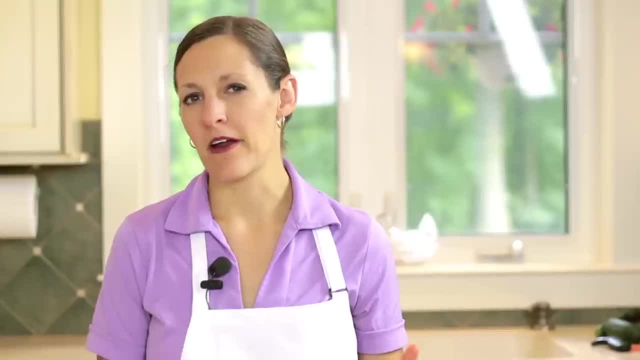 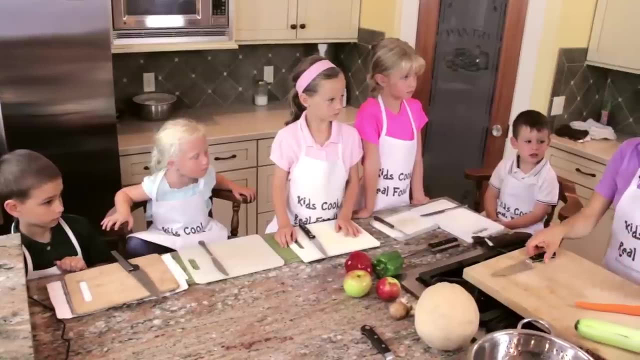 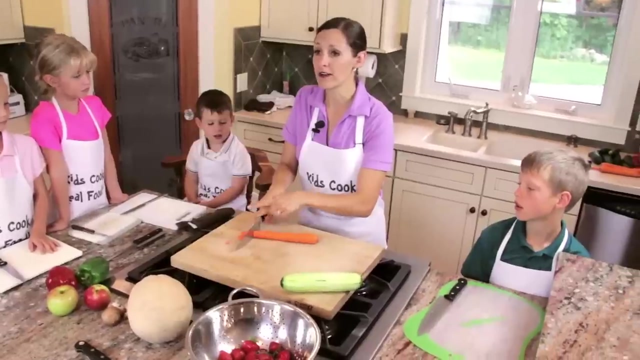 I want everybody to remember, and I'm trying to make it really easy to remember: Knife moves eyes down. Food moves knife down. What that means is, if you are cutting away, your eyes need to be looking down. If you look up, your knife stops moving and 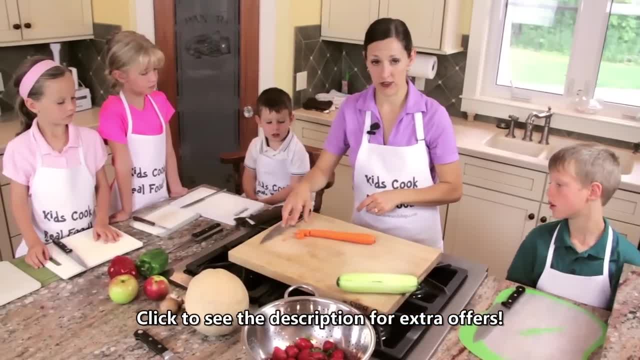 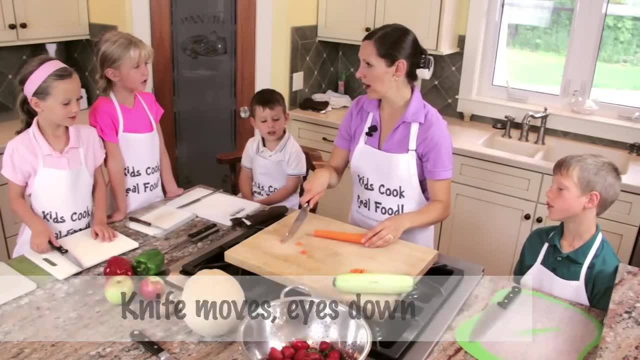 then when you need to move your food to the plate, the knife goes down because the food is moving. Okay, guys, Can you say that with me? Say: knife moves eyes down. Ready, Let's try it again. Ready, Say-. 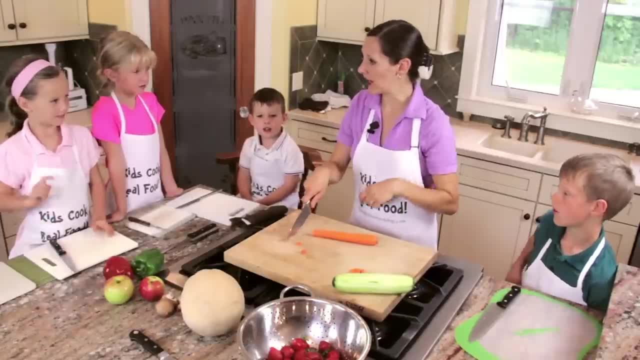 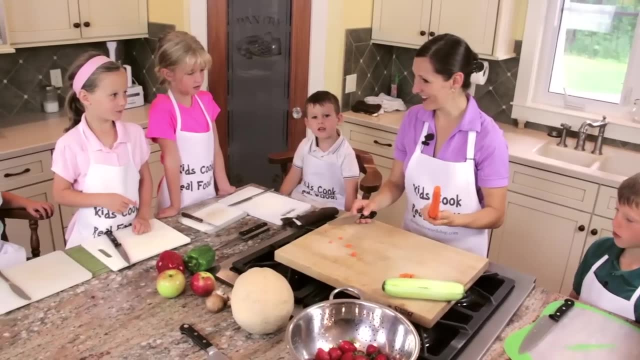 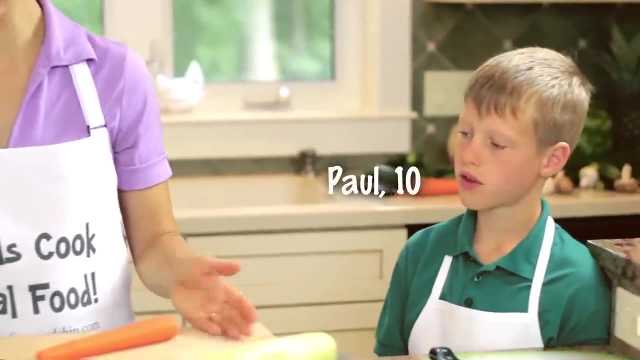 Knife moves eyes down. Great συν multiplier for aus- Knife moves, eyes down. All right, now say: food moves, Food moves, Knife down, Knife down. Let's do it all together ready. Food moves, knife down. 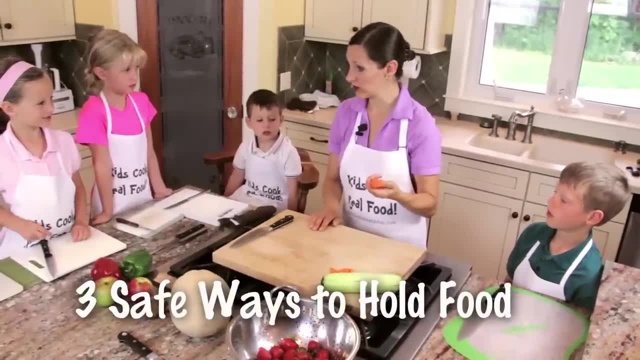 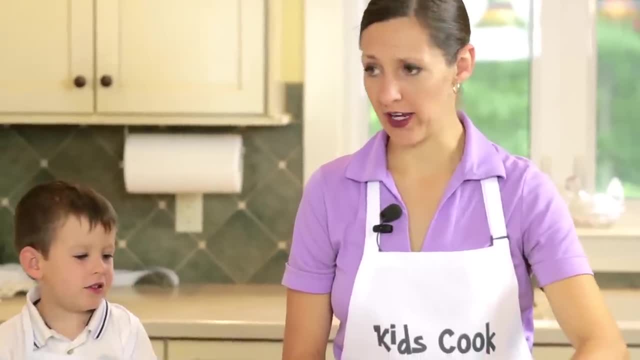 Now we're gonna talk about the different ways to hold the food, because we want to cut the carrot right, Not the Finger, Not the finger. Sometimes kids hold food like this: Uh-oh, Oh, oh, oh, Pick me, pick me. 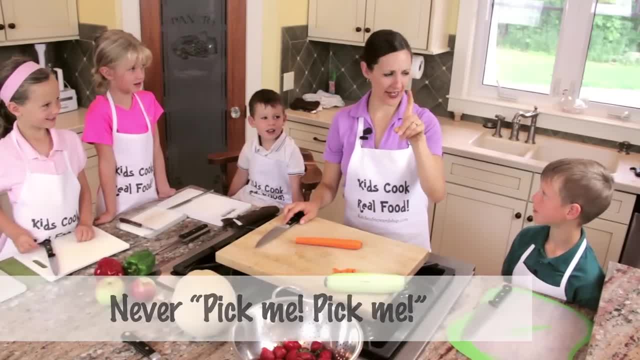 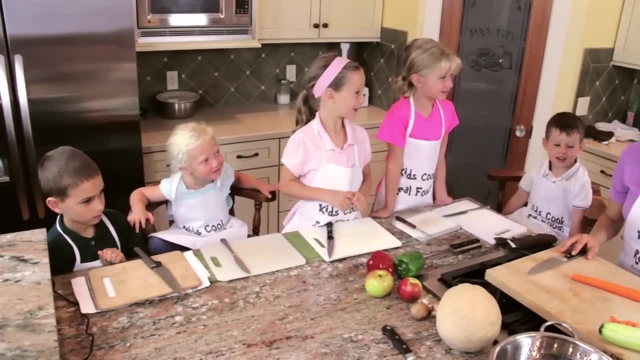 Right, we say that finger's saying pick me, pick me. I want to get cut. Yikes, We don't want to do that, right? So you shake your head and go. no way, We don't want to do pick me, pick me. 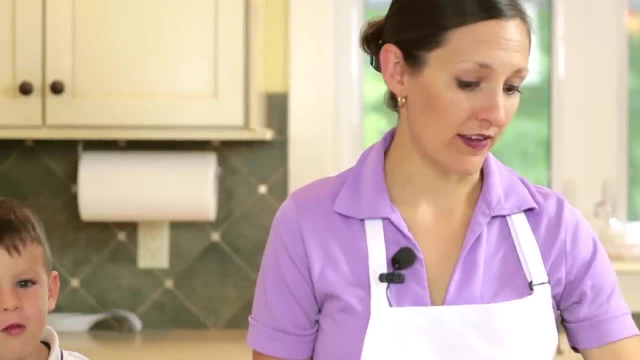 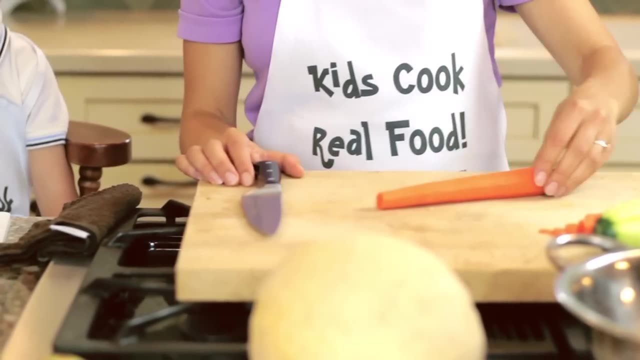 So your adult guide is going to remind you. if they see fingers pointing toward a sharp knife, they're going to say, pick me, pick me. And that means, oh, you need to get down to the other end. We're going to stand our fingers up like this: 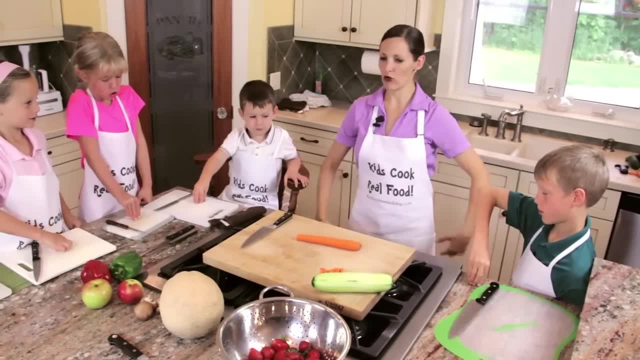 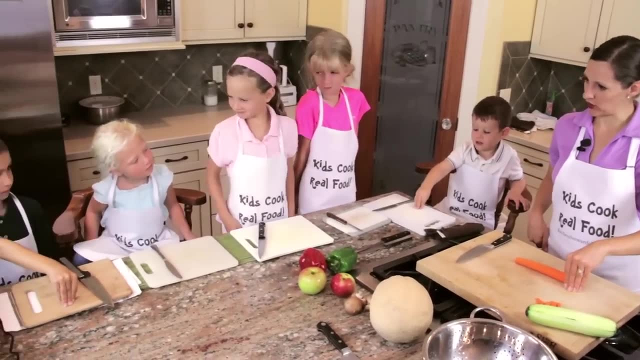 Can everybody stand your fingers up really straight on your board, Right, like a soldier stands at attention, like that? Oh, that's very good, girls. Like a soldier standing at attention. So that's what your fingers do, because you know what. 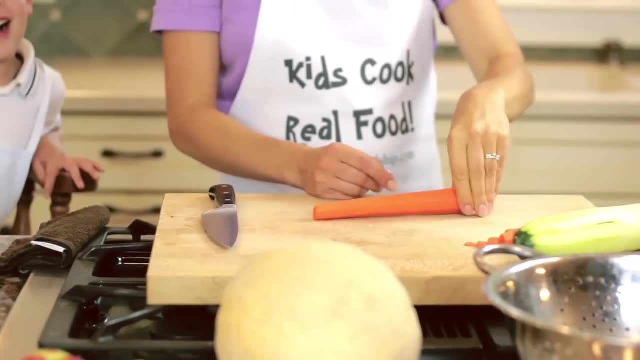 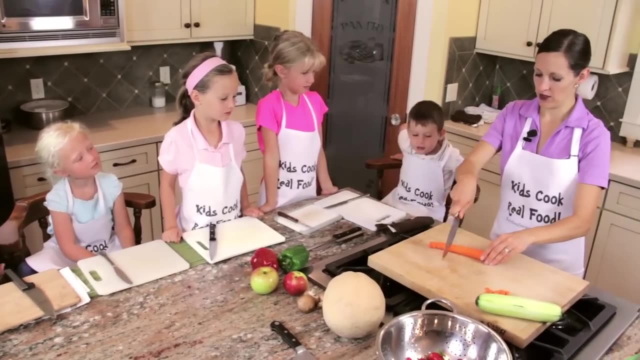 Then they're not standing out, going pick me, pick me. So they're going to stand at attention And I say hey, hey, out of the way, Get all the way to the end right Now. sometimes we're going to cut different ways. 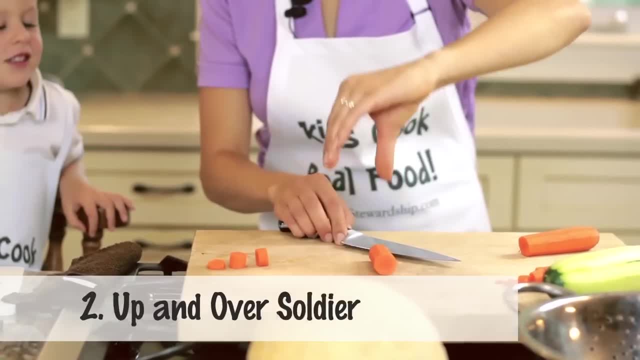 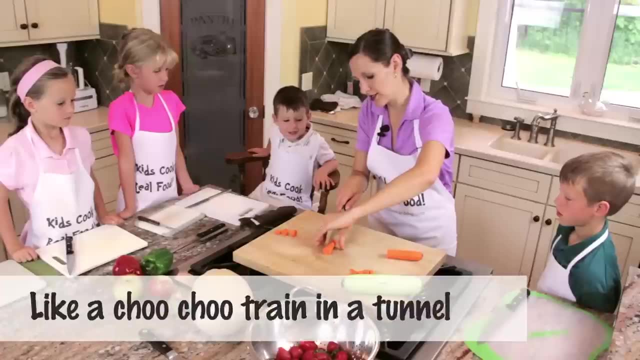 So we've got another way to get soldiers and it's like this kind of like a tunnel. We call it up and over soldier. Fingers are still standing up, but the knife chugga, chugga, chugga, chugga, choo choo. 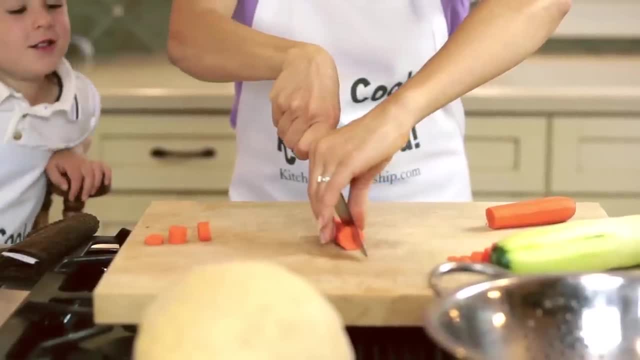 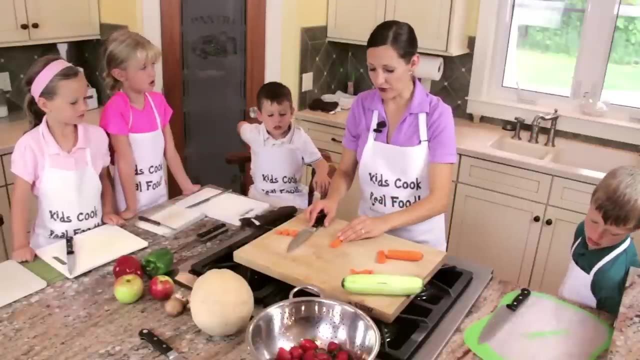 is going to go through that tunnel just like a train And it's still going to be super safe. My fingers are still far away from the knife. They're standing up. It's called up and over soldier. The last way to hold the food is not really holding the food. 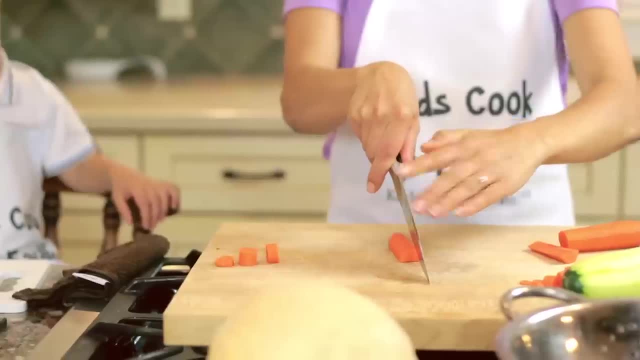 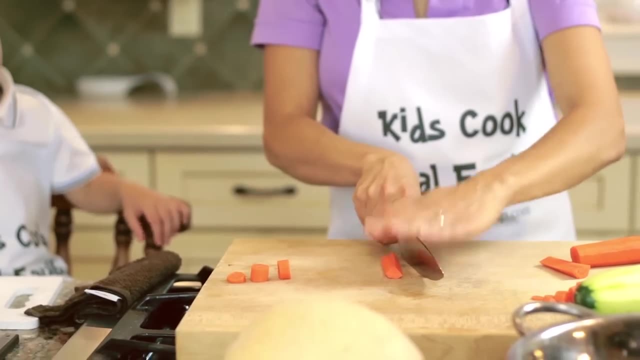 It's helping on the knife. So sometimes we put our hand on top of the knife. We know that it's not anywhere near the sharp part And we can give a little bit of push to help it along. We're going to call that top chop. 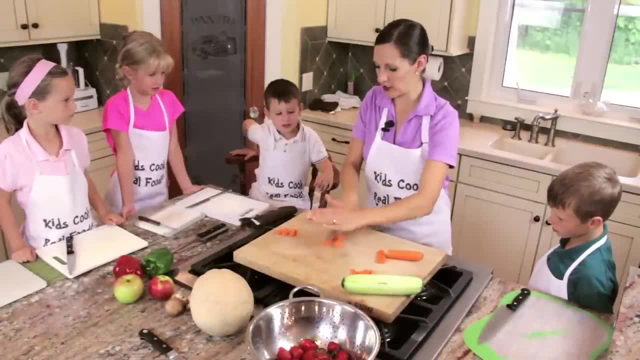 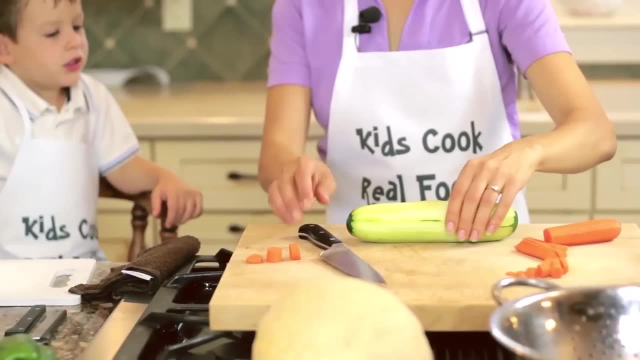 Top chop. yep, because your hand's on top while you're chopping. So we've got three ways to hold the food right. Long piece of food here. We're going to go, hey, hey, out of the way. We're going to go, sometimes up and over soldier, like that. 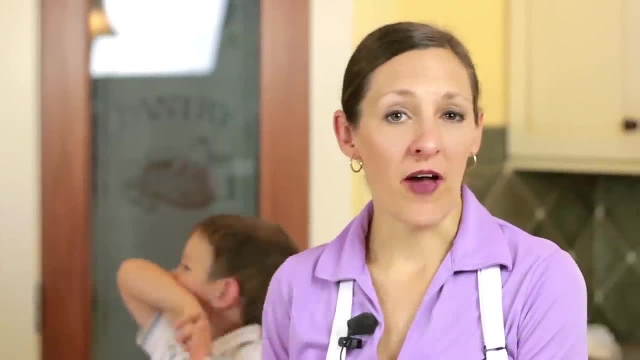 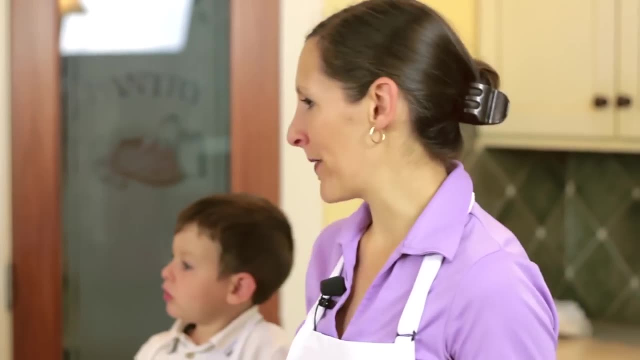 Or we might go top chop. We're going to talk about four different ways to move the knife to chop food, And they're all pretty fun. The first one's like Rockabye Baby. You guys know that song, Rockabye baby. 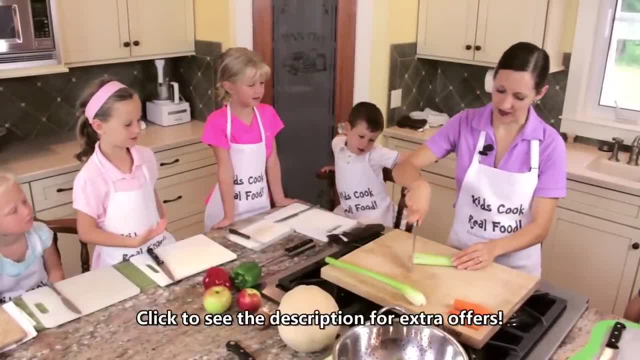 But we're going to rockabye our knife, all right. So let's sing Rockabye Knife, And that means I'm just going to kind of rock the knife up and down. The knife tip is always, always, always touching the board. 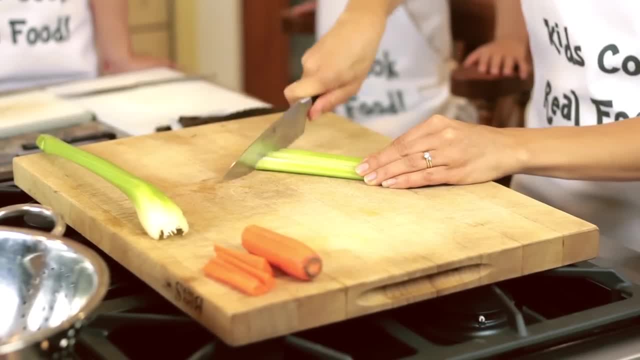 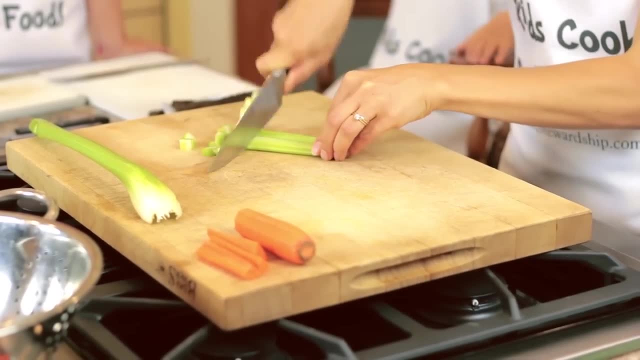 It is not going to move, Just my hand will move up and down. ready Rockabye knife in the celery. And oh, I got to move those hands down and get them up like a soldier. Now set the knife down and I can move the food. 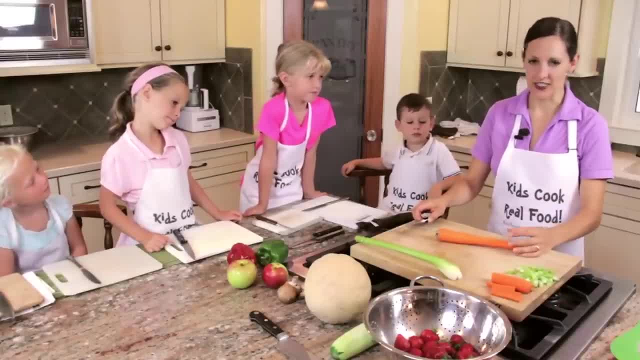 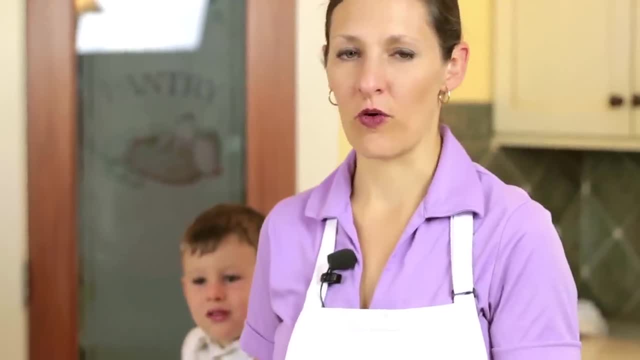 The second way we're going to talk about cutting with our knife is driving it like a vacuum. So when you vacuum, you push back and forth, back and forth, And this is good also for kind of like when I did with the celery and with a carrot. 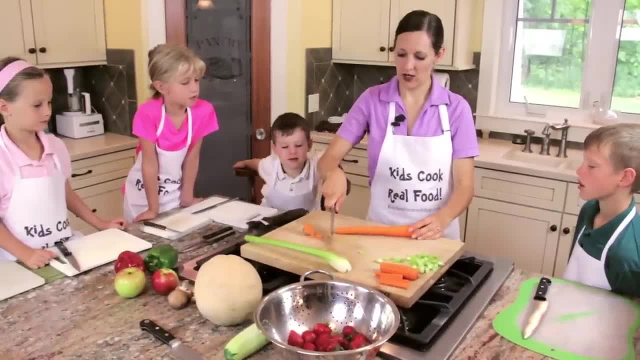 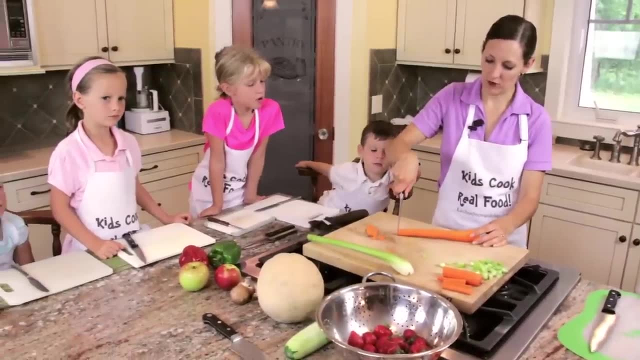 Let me turn this carrot around here. We're going to cut little wheels of our carrot, But instead of just going up and down, I'm going to drive like a vacuum. The knife tip stays on the board like that And I cut on my way forward, back and back and forth, back. 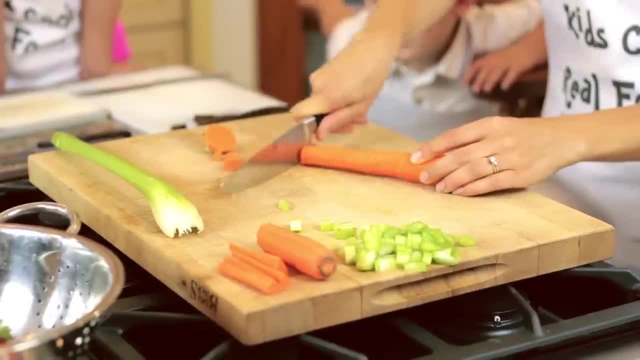 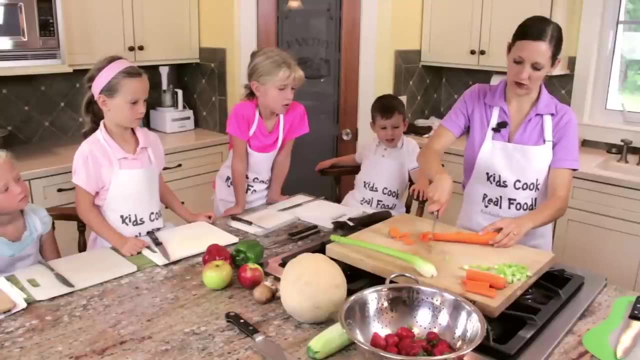 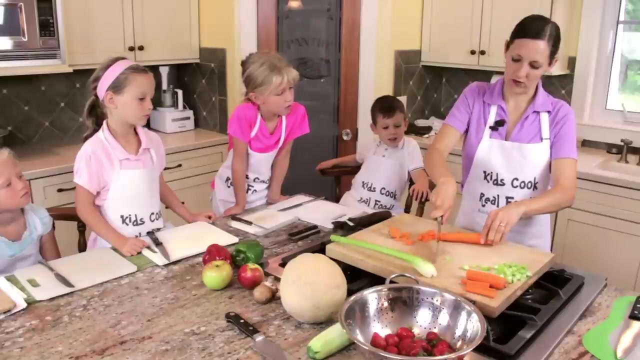 and forth. So we're kind of driving it like a vacuum and sliding it back and forth, But notice, my knife never comes up, because then I start to lose control. It's really, really controlled when I can slide it back and forth, back and forth. 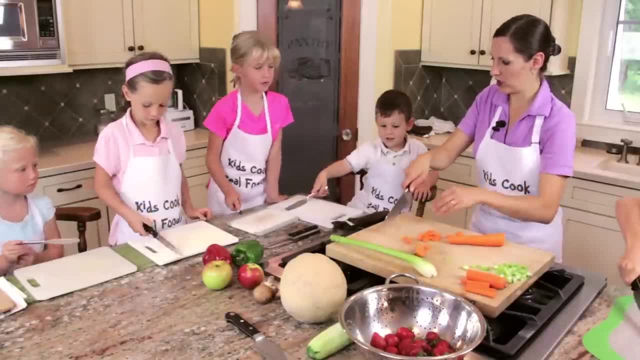 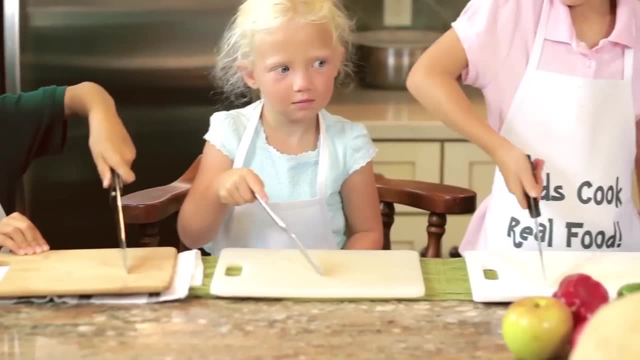 Everybody. pick up your knife. Let's try that one. Put your tip on the board and just drive it forward, back forward, back forward, back. Leah, you got to turn your hand a little bit because your thumb isn't right on top. 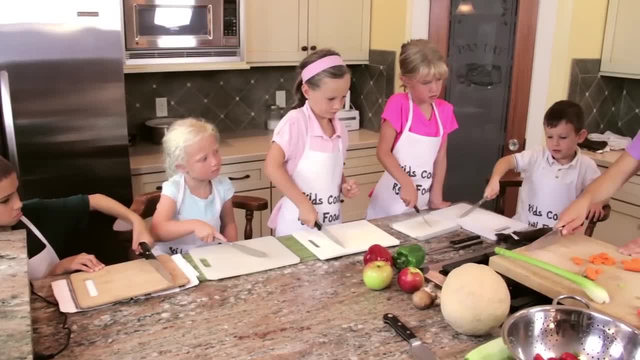 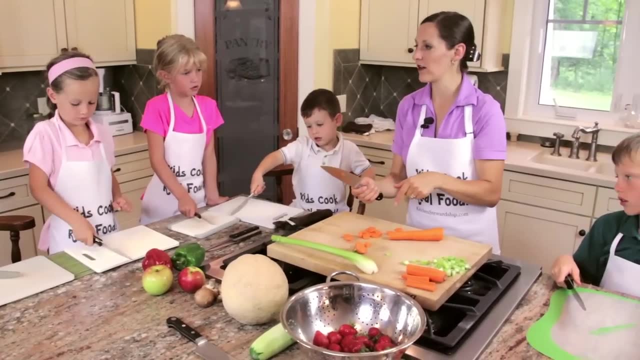 Yeah, your hand should be on top Good Forward, back, forward, back. Now that doesn't really work with little knives like this. It's better with this nice curved chef's knife, But it's still fun to kind of practice. 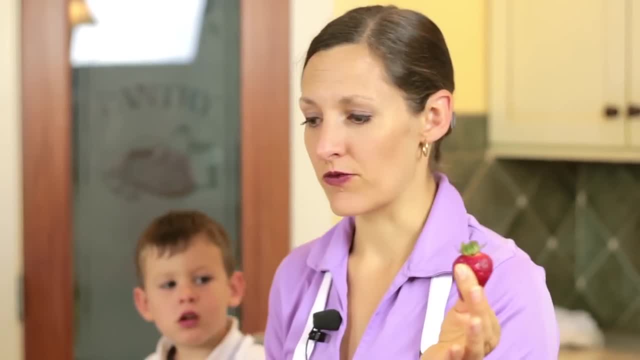 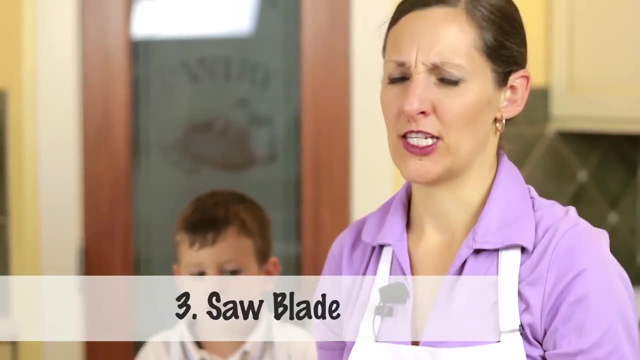 Knife. strategy number three is for soft foods like strawberries or big things like melons, And we're going to call this one saw blade. In fact, I may even grab a smaller knife for my berry Saw blade. It's just how it sounds. 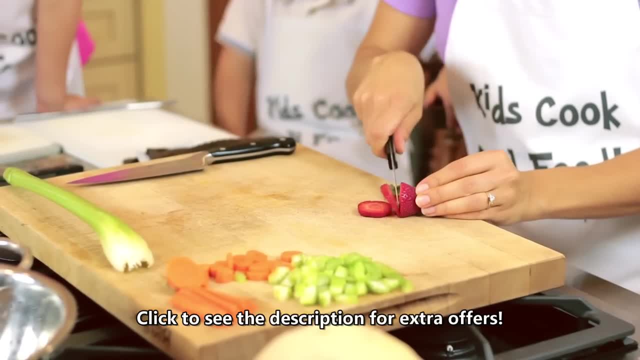 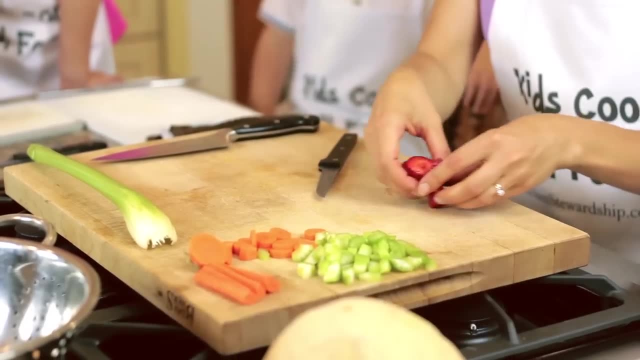 You saw back and forth And it's great. I mean, this strawberry is really really soft. Notice, my tippy fingers are hey, hey out of the way I set the knife down and I move my food. So saw blade is also great for these big, huge things. 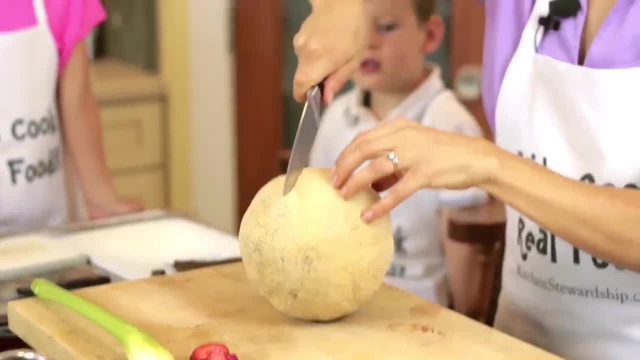 I'm going to poke it just a little so that I get in the right spot. Hands are out of the way And I'm going to zhugga, zhugga, zhugga, right, We're just going to saw right through that. 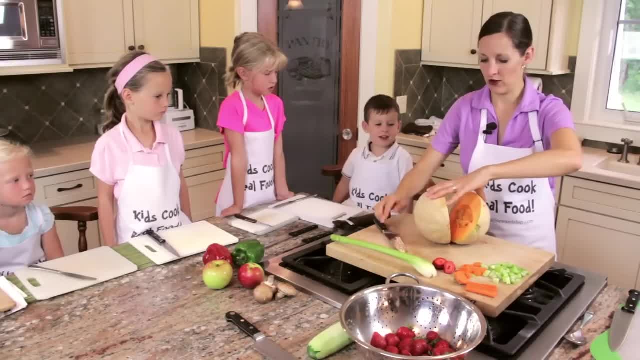 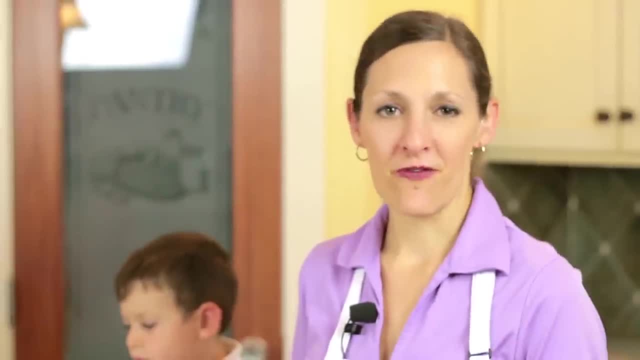 And I'm making sure always my hands are out of the way. Oh, my goodness, Oh smell that. Oh, I just want to eat it. Knife slice number four is called the tug-a-war pull And this is for slicing, mostly for little things. 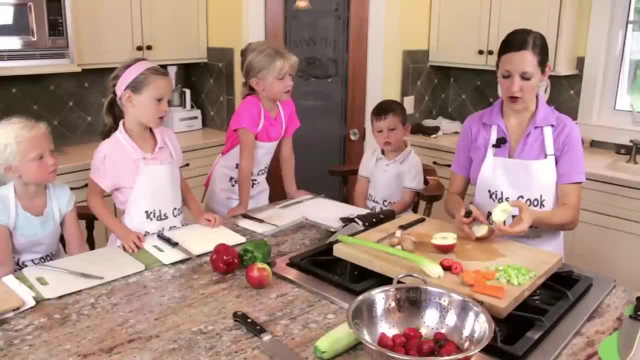 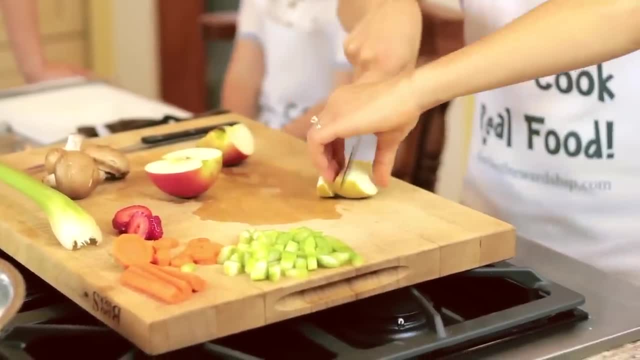 kind of with a smaller knife. So I've got here an apple that I've taken the core out And it's called quartering, And I'm going to do the up and over soldier hold And then I'm going to pull my knife through the apple. 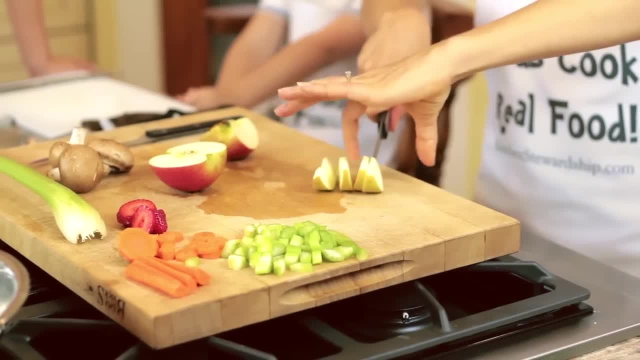 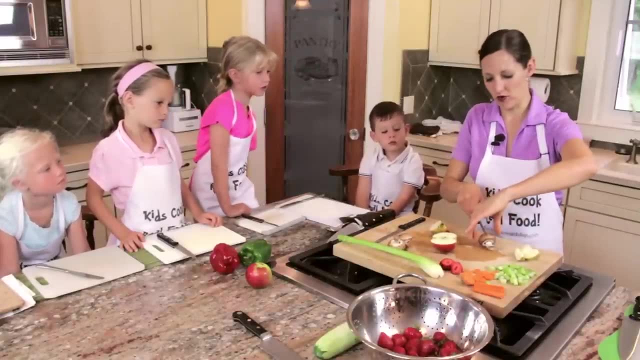 Pull it through, Pull it through. My fingers are completely far away from the blade And I'm just pulling it through. I can do the same thing with something soft and small like a mushroom. Up and over, soldier, hold tug-a-war, pull, slice, slice. 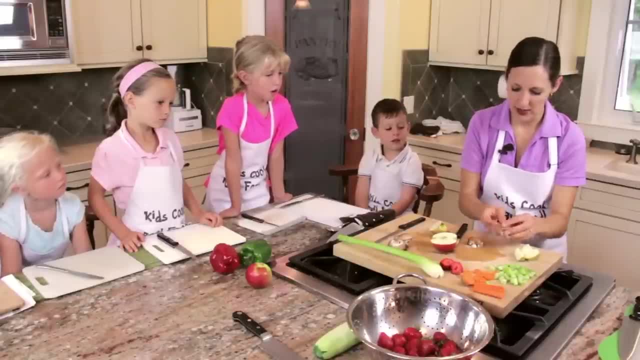 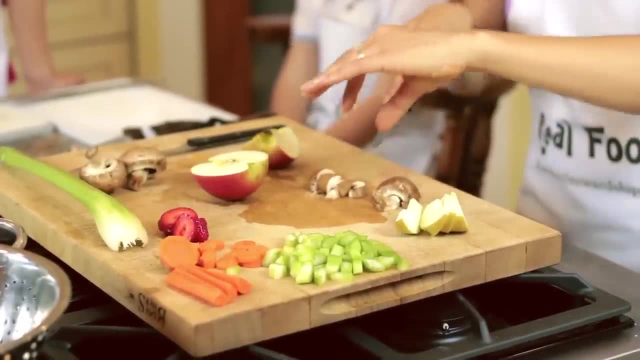 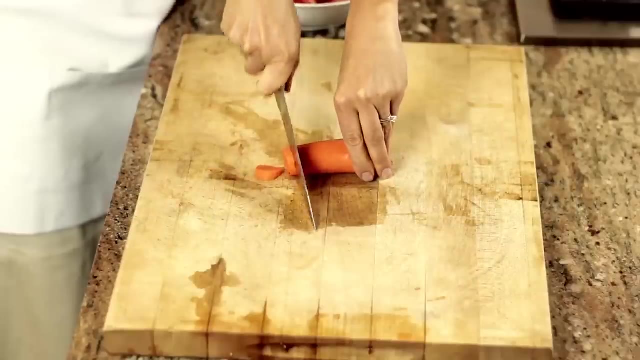 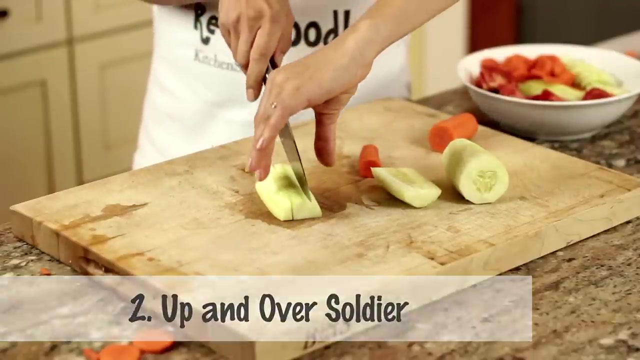 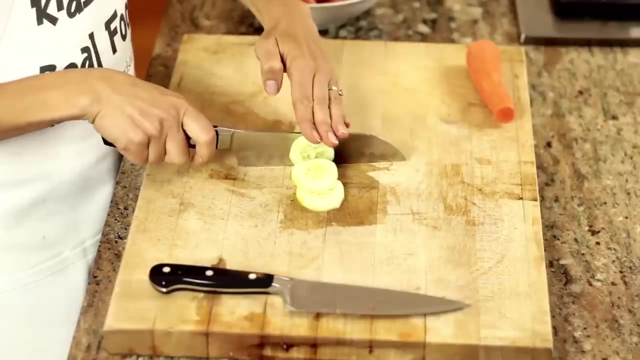 right, And then I can take that mushroom and lay the flat sides down And I can cut it even smaller and kind of go over top, pull it through, And then I can do just the same thing. It's just sort of pulled through. 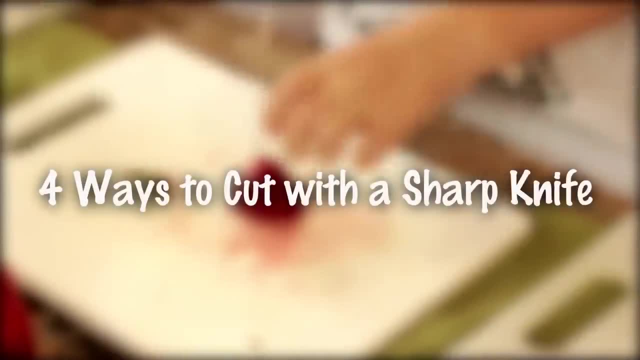 And then I can do that. I can pull my knife like this, and then I can get a big mushroom And then I just pull it through and then it's up and over right, And then I can just pull it through. 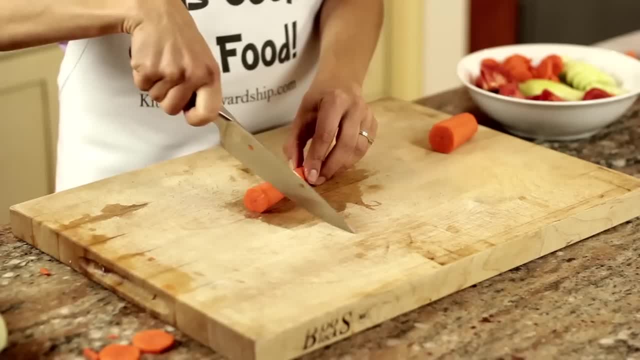 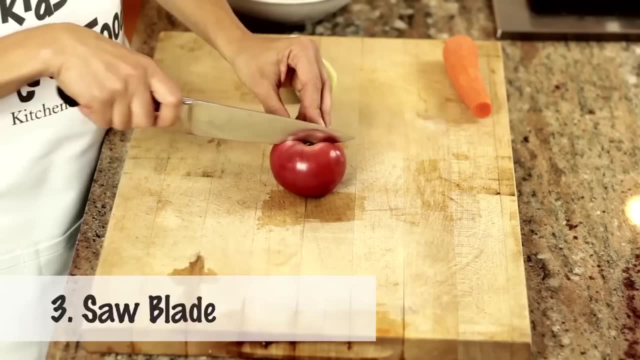 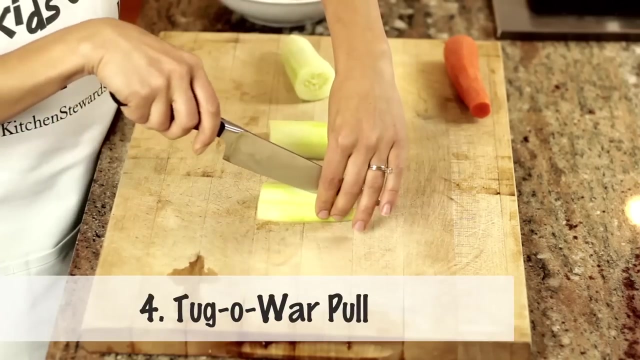 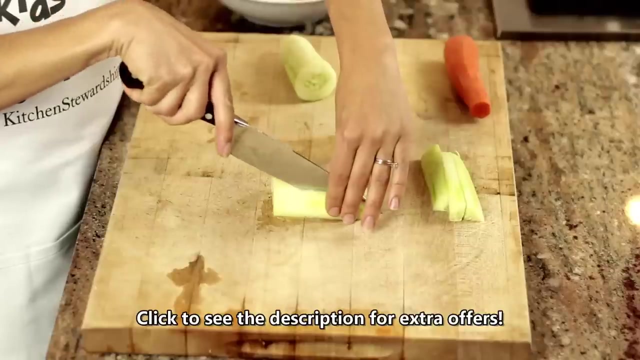 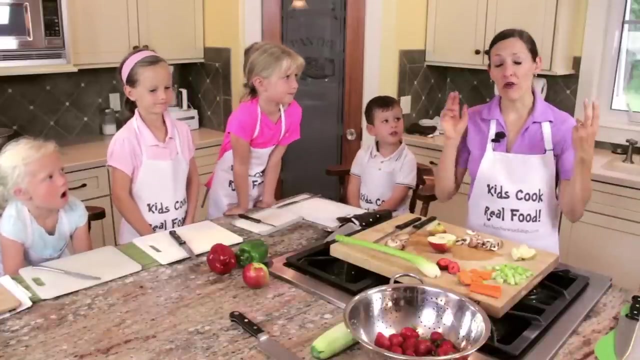 Up and over soldier, hold tug-a-war, pull slice, slice, slice, Pull it through, Pull it through, Pull the knife through. It's tough when you do it like that, Yeah, And then I do something, All right. so now you know three safe ways to hold food, four ways to move your knife.